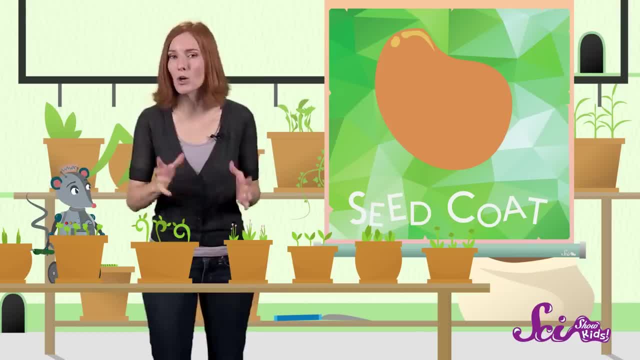 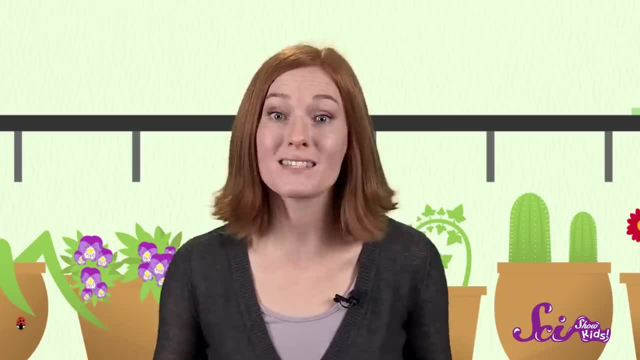 plant inside and keeping it from drying out. The seed coat also has super-sensing powers. It has special chemicals in it that can tell when the seed is in the right place to start growing. For example, the sunflower seeds and the pumpkin seeds in your trail mix. sense that it's. 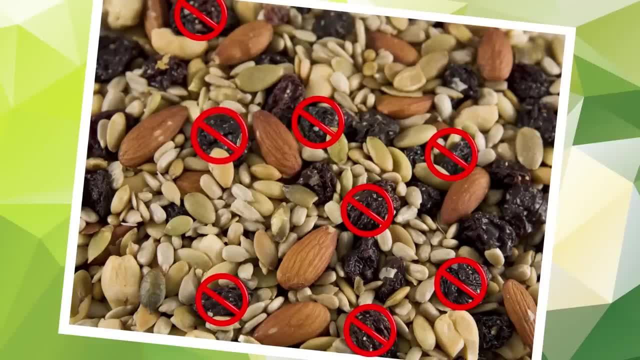 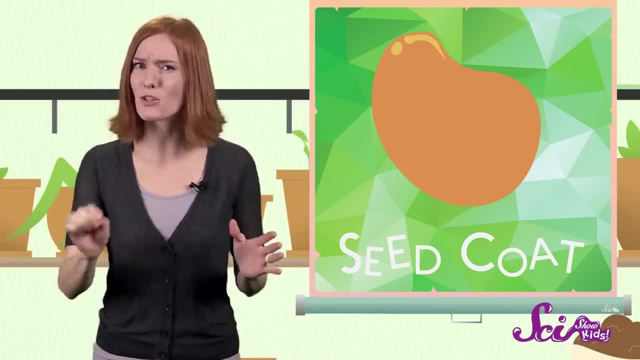 not safe to grow. After all, seeds can't grow when they're surrounded by raisins and chocolate chips. So while the seeds are in a bag or in your hands, it's like they're asleep. The seeds are still alive, but they're dormant or inactive. Some seeds can stay like this for. 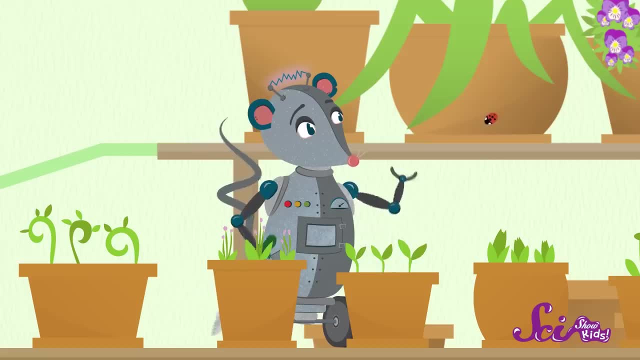 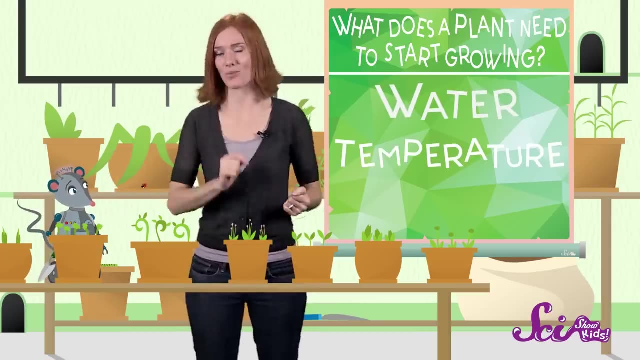 hundreds or even thousands of years. Great question Squeaks. To get started, every seed needs water, the right temperature and the right amount of light. Once the seed has these three things, like when it's planted in some nice wet soil. 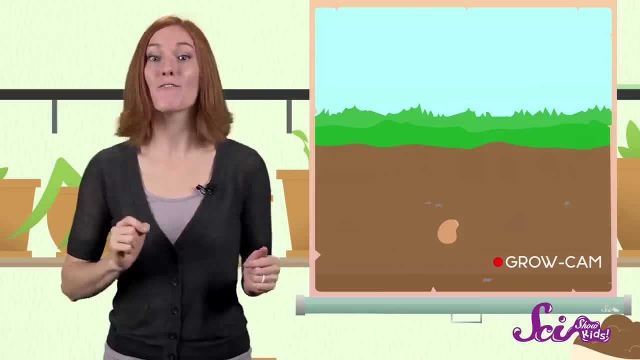 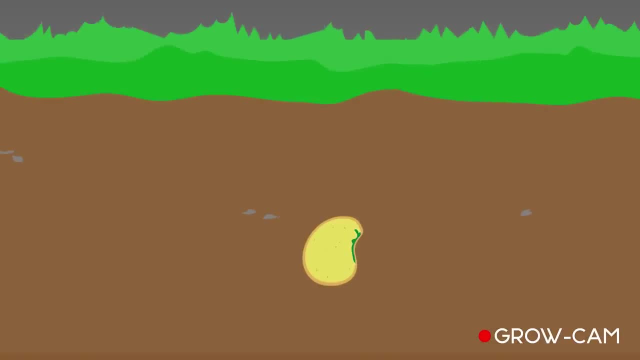 the embryo or baby plant gets the signal to start growing. For plants this growing process is called the embryo. First, the seed coat lets some water through to the embryo. but the embryo needs more than just water if it's going to grow. Good thing, there's a whole bunch of plant food right. 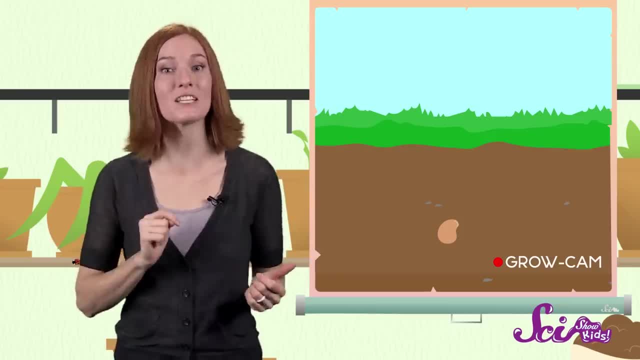 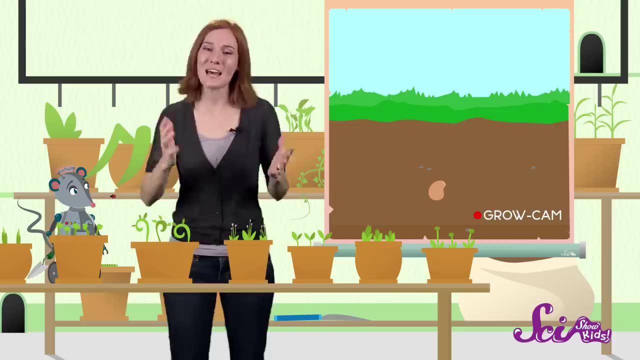 there inside the seed. Until the plant can make its own food from sunlight, which it will need leaves to do. it relies on the endosperm for energy. It's like the little baby plant has its own backpack of snacks, So the embryo keeps growing and taking in more water until the seed coat cracks open. 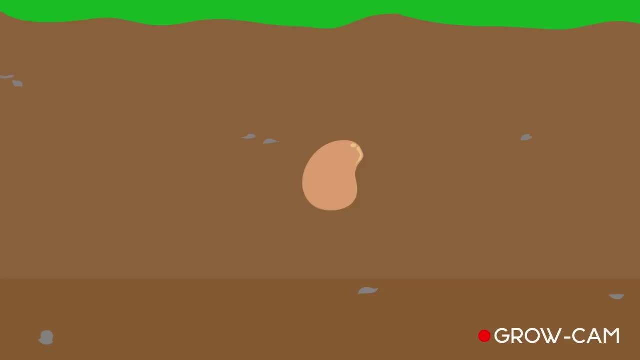 and the embryo kicks out a kind of a foot, But not at all like my foot. The first part of the seed is the root. The root always grows downward, no matter what way the seed is planted. A seed can actually tell which way is up and which way is down, so the root pushes down deeper and deeper. 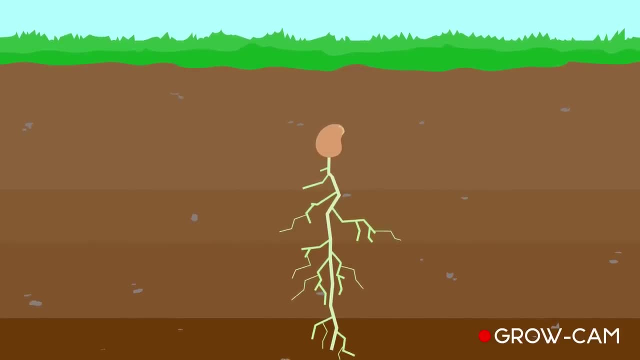 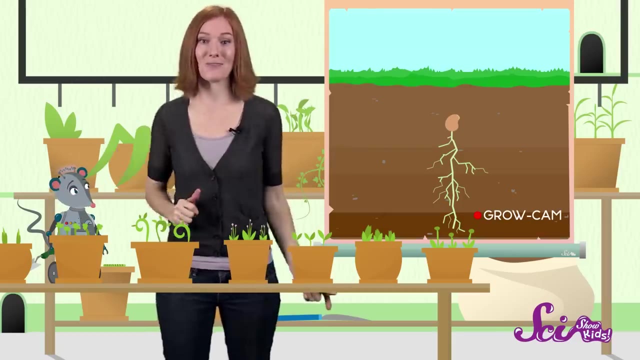 into the soil, looking for more water and minerals to feed the baby plant. Once the plant is all grown up, those deep roots will have another job. They'll help keep the plant from falling over or blowing away in the wind. But soon after the first baby root finds its way into the dirt, another part of the seed 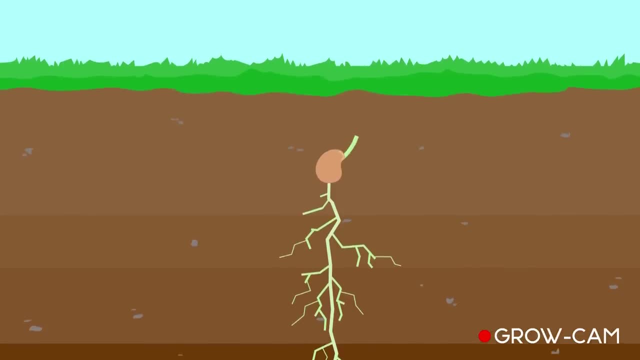 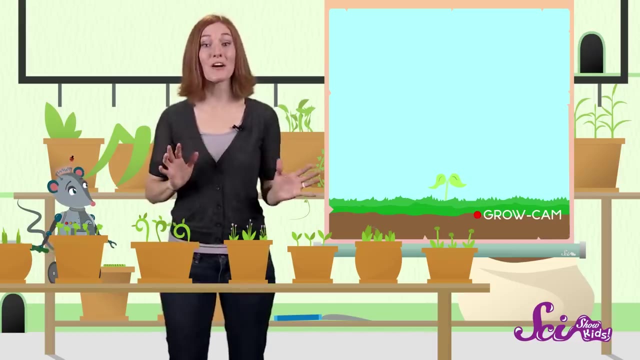 pops out, this time in the opposite direction. A shoot, which happens to be a seed that's growing up, has the stem of the plant and a few leaves pushing its way up towards the sunlight. Once the shoot breaks through the soil to the open air above, we say that it's sprouted. 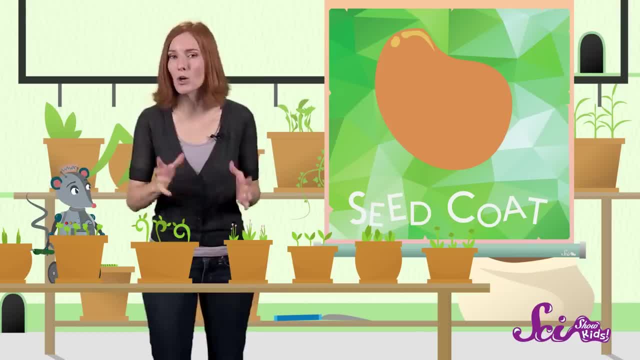 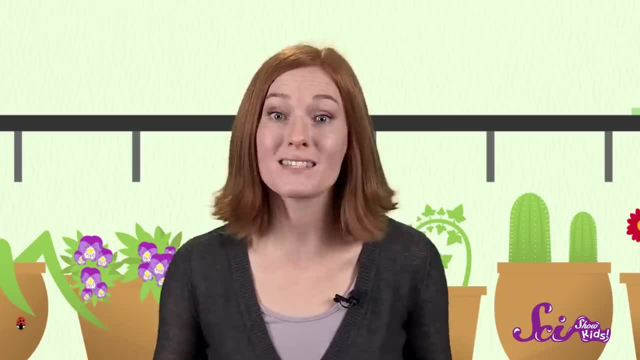 plant inside and keeping it from drying out. The seed coat also has super-sensing powers. It has special chemicals in it that can tell when the seed is in the right place to start growing. For example, the sunflower seeds and the pumpkin seeds in your trail mix. sense that it's. 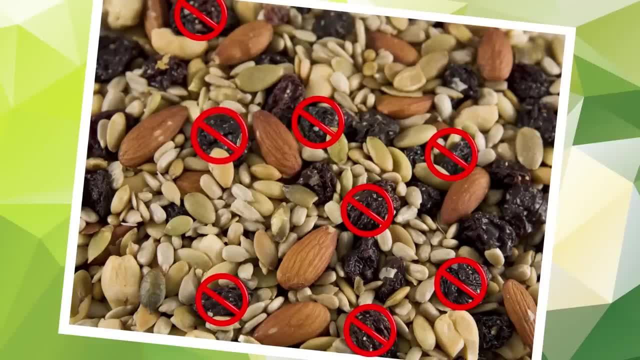 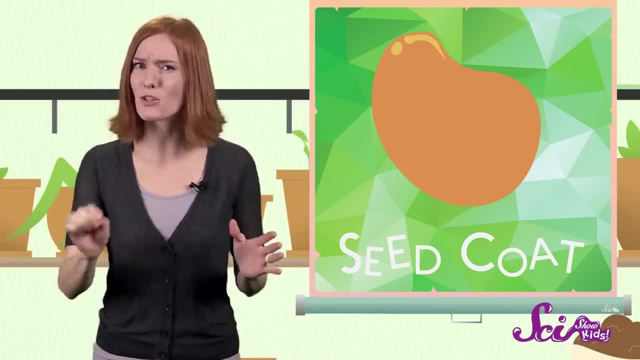 not safe to grow. After all, seeds can't grow when they're surrounded by raisins and chocolate chips. So while the seeds are in a bag or in your hands, it's like they're asleep. The seeds are still alive, but they're dormant or inactive. Some seeds can stay like this for. 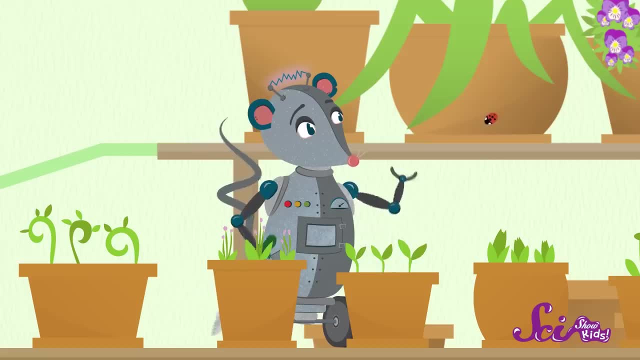 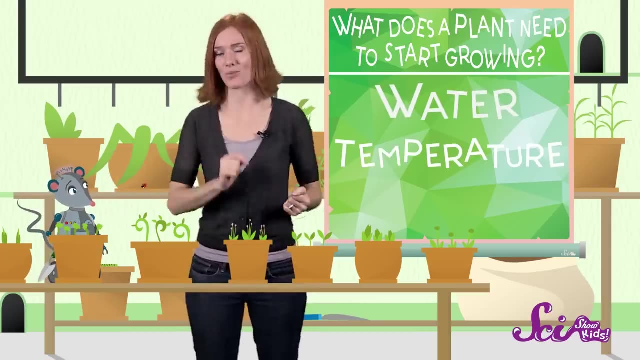 hundreds or even thousands of years. Great question Squeaks. To get started, every seed needs water, the right temperature and the right amount of light. Once the seed has these three things, like when it's planted in some nice wet soil. 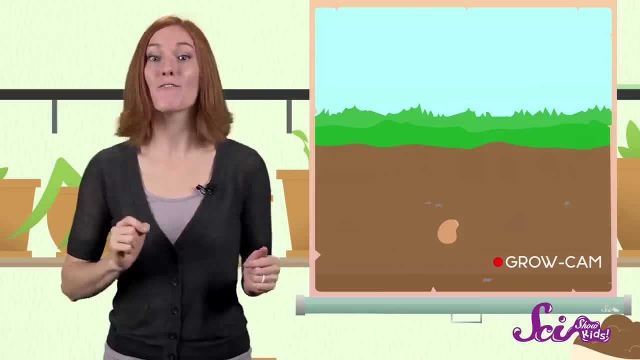 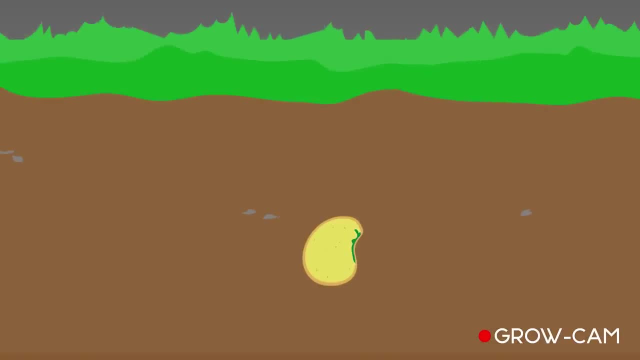 the embryo or baby plant gets the signal to start growing. For plants this growing process is called the embryo. First, the seed coat lets some water through to the embryo. but the embryo needs more than just water if it's going to grow. Good thing, there's a whole bunch of plant food right. 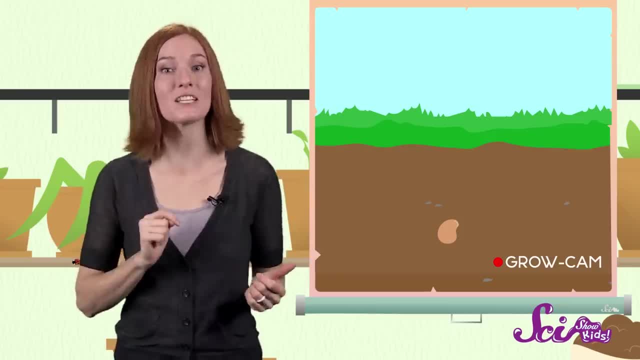 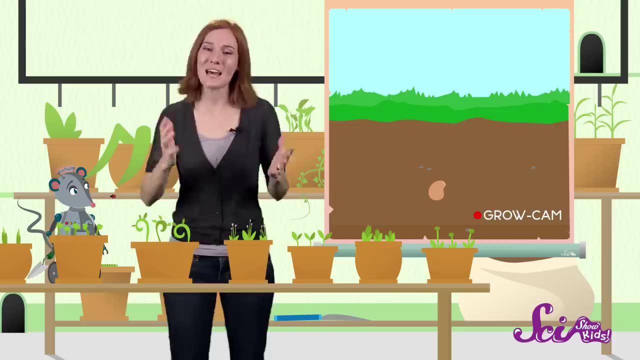 there inside the seed. Until the plant can make its own food from sunlight, which it will need leaves to do. it relies on the endosperm for energy. It's like the little baby plant has its own backpack of snacks, So the embryo keeps growing and taking in more water until the seed coat cracks open. 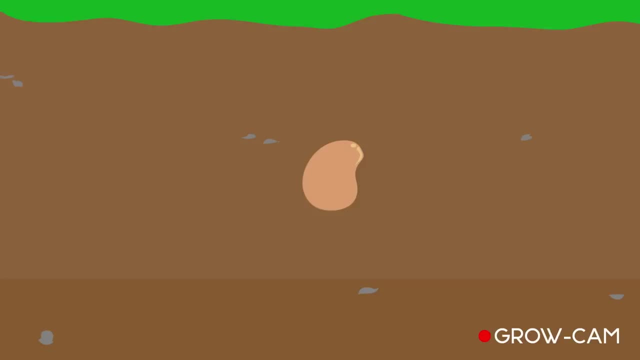 and the embryo kicks out a kind of a foot, But not at all like my foot. The first part of the seed is the root. The root always grows downward, no matter what way the seed is planted. A seed can actually tell which way is up and which way is down, So the root pushes down deeper and deeper. 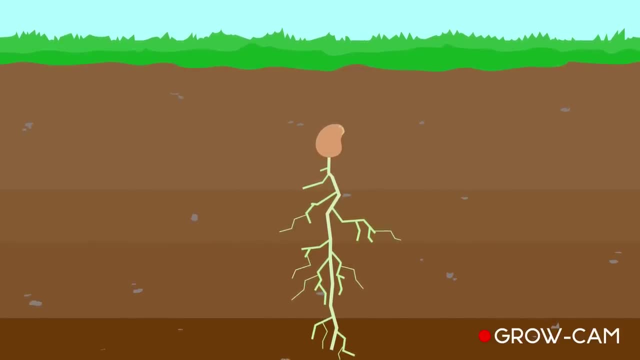 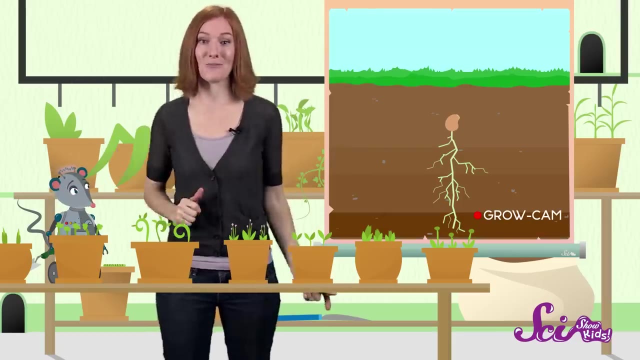 into the soil, looking for more water and minerals to feed the baby plant. Once the plant is all grown up, those deep roots will have another job. They'll help keep the plant from falling over or blowing away in the wind. But soon after the first baby root finds its way into the dirt, another part of the seed 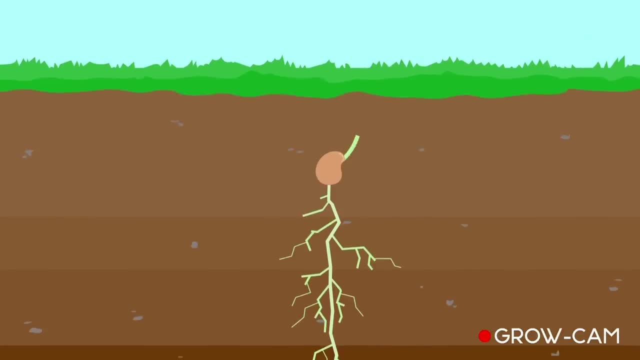 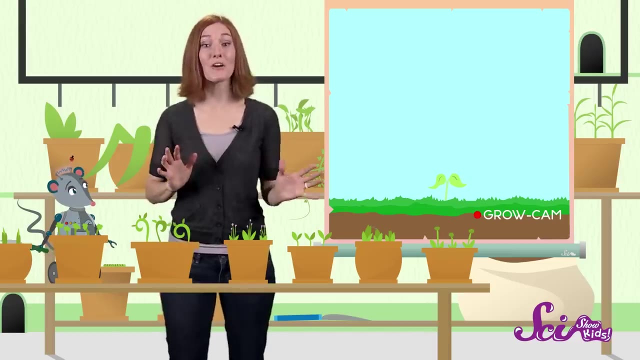 pops out, this time in the opposite direction: A shoot. It has the stem of the plant and a few leaves and pushes its way up towards the sunlight. Once the shoot breaks through the soil to the open air above, we say that it's sprouted.